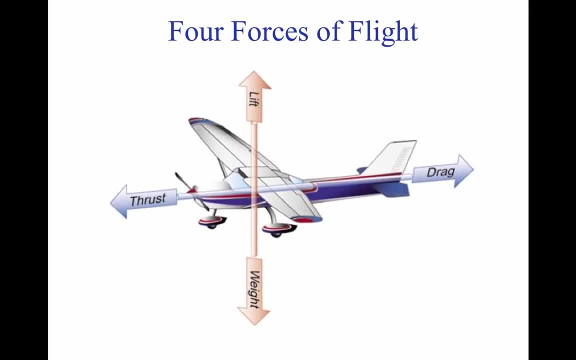 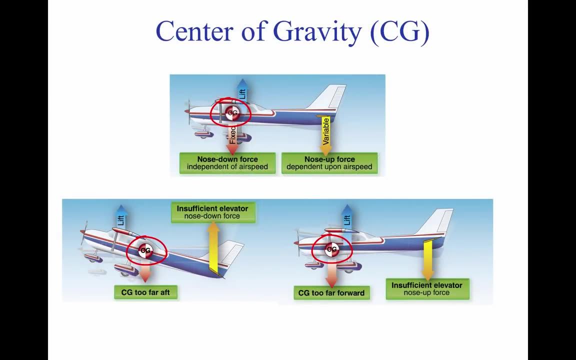 Lift and weight always act through the airplane's center of lift and center of gravity respectively. Center of gravity is the point on the aircraft in which, if the airplane were suspended, it would remain level. The position of the center of gravity is very important for aircraft. 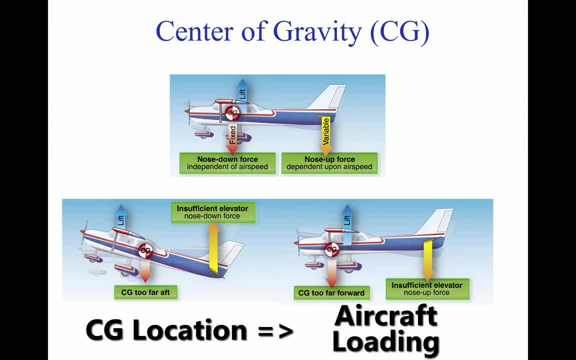 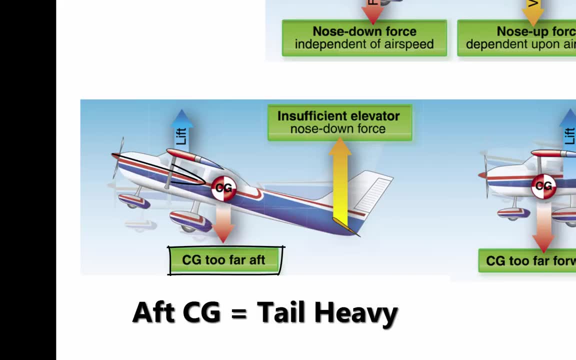 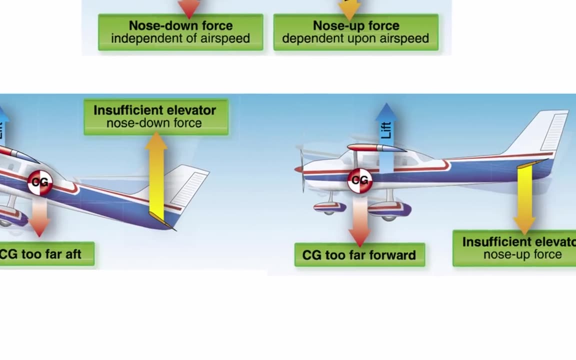 and can be affected by the installation of onboard equipment, aircraft loading and other factors. When the center of gravity is too far- aft, far towards the rear of the aircraft, the plane will have a tendency to pitch up, which can cause the plane to stall, While having the center of gravity too far forward, the 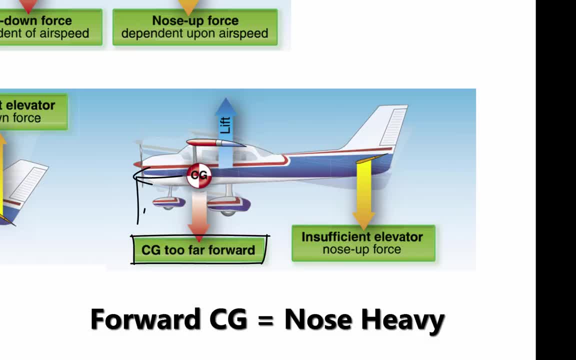 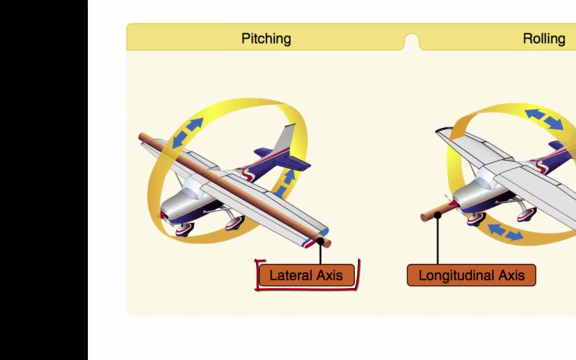 plane will have a hard time getting off the ground and the nose will tend to pitch down. Aircraft move around three different axes. The lateral or pitch axis is a line drawn from the wingtip through the plane's center of gravity to its other wingtip. The longitudinal 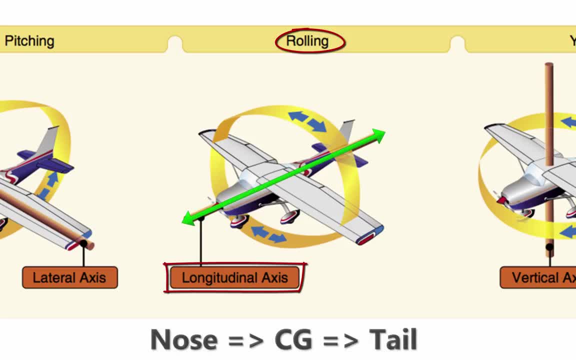 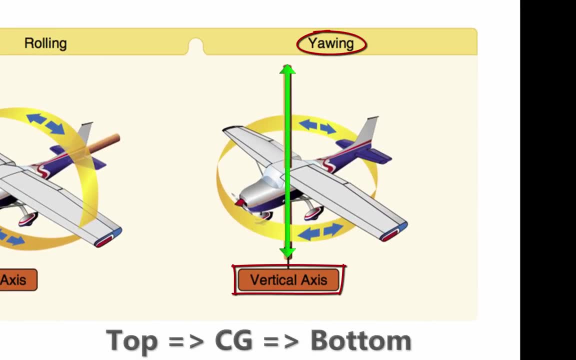 or roll axis, is drawn from the nose to the tail of the aircraft, again passing through the center of gravity, and the vertical or yaw axis is drawn vertically down through the plane's center of gravity, Although airplanes are designed for a variety. 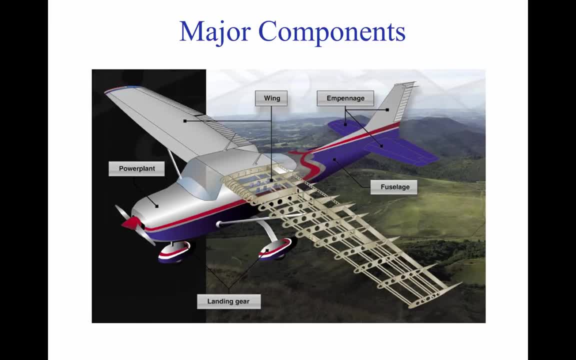 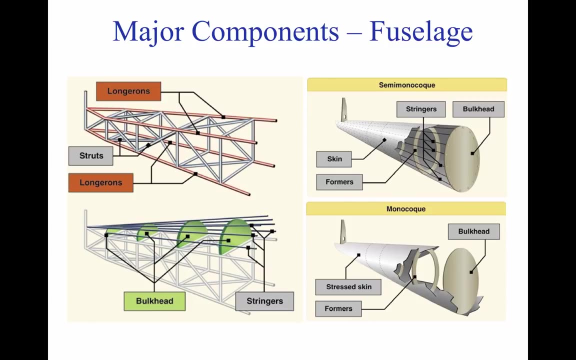 of purposes, most of them have the same major components. Most airplane structures include a fuselage, wings, an empennage, landing gear and a power plant. The fuselage is the central body of an airplane and is designed to accommodate the crew, passengers and cargo. 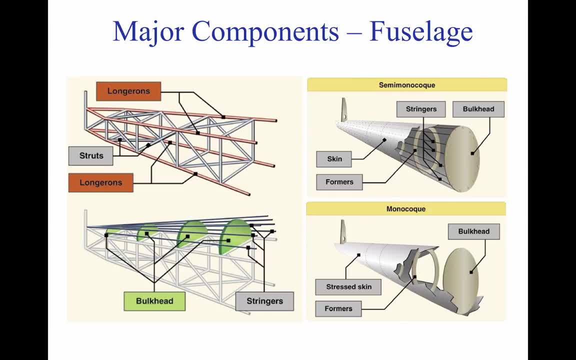 It also serves to connect all the other main components of an aircraft Pictured above. have there three different types of fuselage structure: trusts, semi-monocoque and monocoque. There are many different flying class sizes on the fuselage structure, including tresondos. 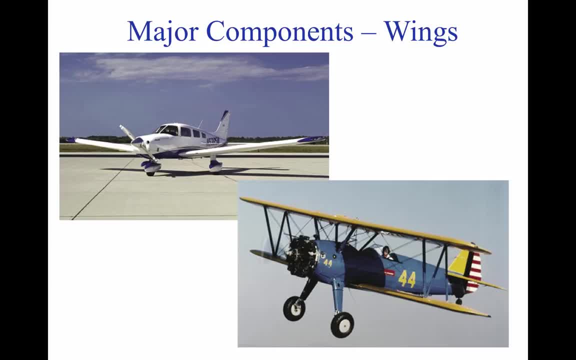 different designs, shapes and sizes of wings used by the various manufacturers. However, their main purpose is to lift the plane into the air. Above are two different designs. The plane in the upper left has one wing and is called a monoplane. 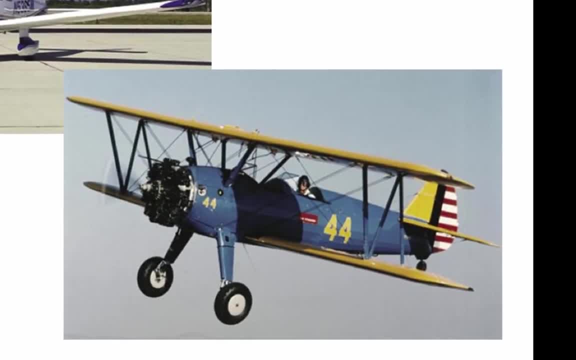 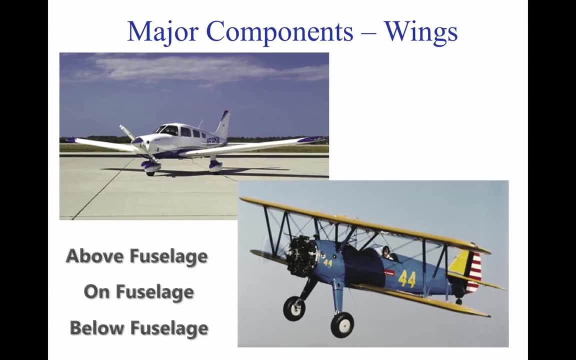 The plane in the lower right has two wings, referred to as a biplane. Wings can be placed above, on and below the fuselage. These different wing placements are referred to as high-, mid- and low-wing planes. Most high-wing planes have external struts to help dissipate the wing's load to the rest of the plane. 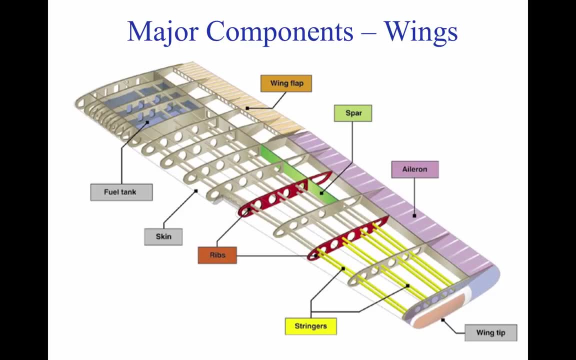 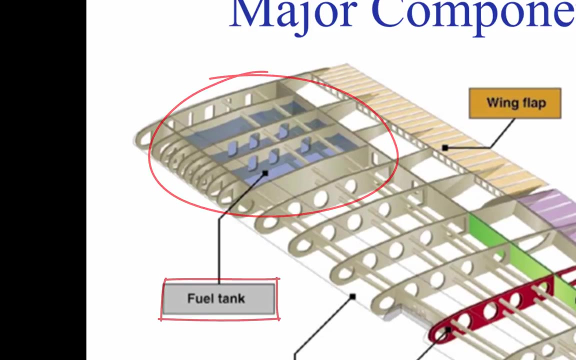 The picture above shows the general construction of a modern wing. The ribs, stringers, spar and skin all give the wing structure. The fuel tanks in most modern airplanes are also contained in the wing, near the fuselage, as part of the wing or in flexible containers. 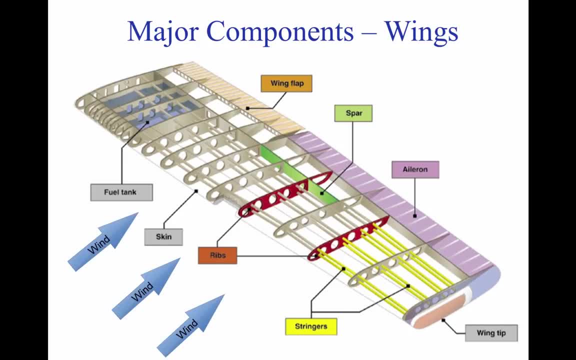 The front of the wing is the edge that the wind hits first, also known as the leading edge. Attached to the opposite side of the wing or trailing edge are two control surfaces called the aileron and the flap. Wings are exact mirrors of each other and contain the same control surfaces on both sides of the airplane. 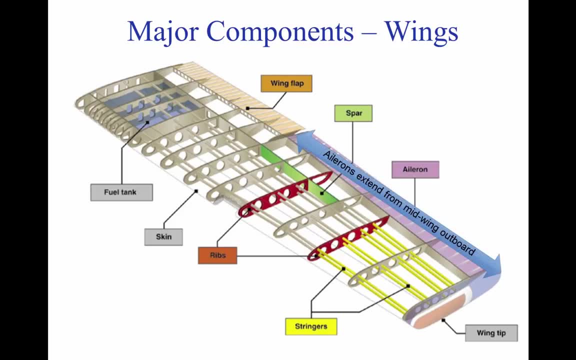 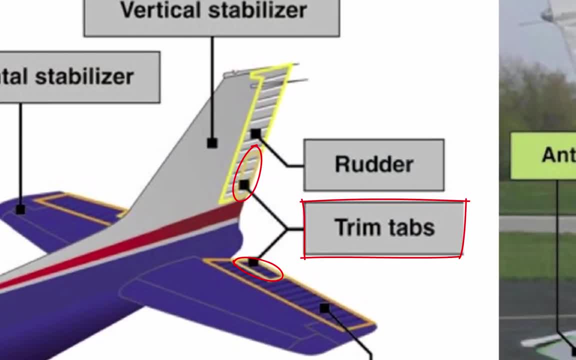 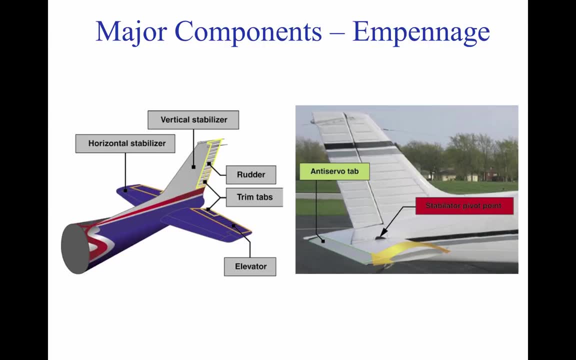 Ailerons extend from about the midpoint of each wing outward toward the tip of the wing. Trim tabs are small movable portions of the trailing edge of the control surface. These movable trim tabs, which are controlled from the flight deck, reduce control pressures. 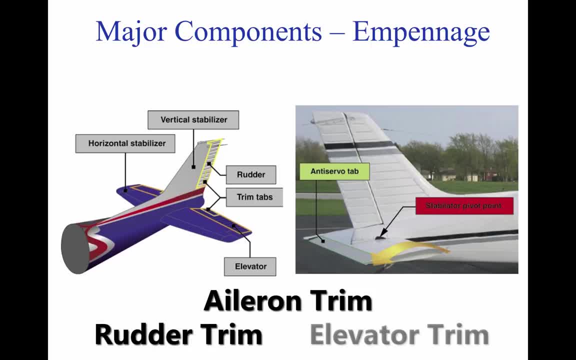 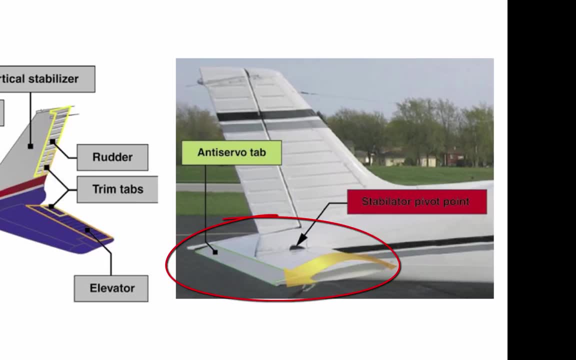 Trim tabs may be installed on the ailerons, the rudder and or the elevator. A second type of empennage design does not require an elevator. Instead, it incorporates a one-piece horizontal stabilizer that pivots from a central hinge point. 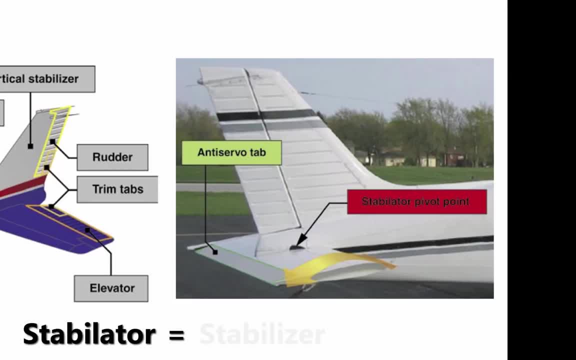 Instead, it incorporates a one-piece horizontal stabilizer that pivots from a central hinge point. This type of design is called a stabilator and is moved using the control wheel, just as the elevator is moved. Stabilators have an anti-servo tab extending across their trailing edge. 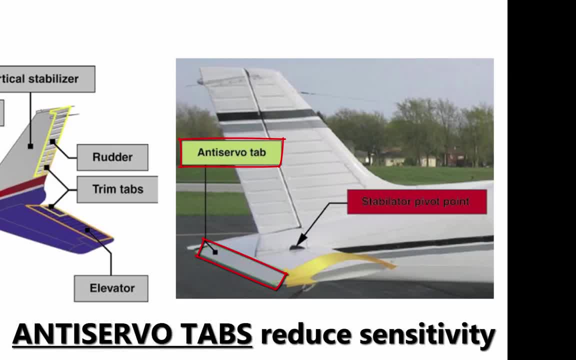 The anti-servo tab moves in the same direction as the trailing edge of the stabilator and helps make the stabilator less sensitive. The anti-servo tab also functions as a trim tab to relieve control pressures and helps maintain the stabilator in the desired position. 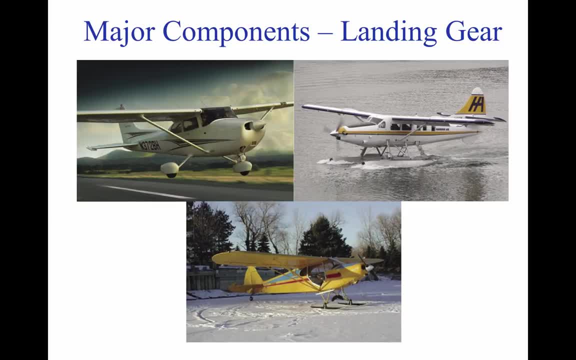 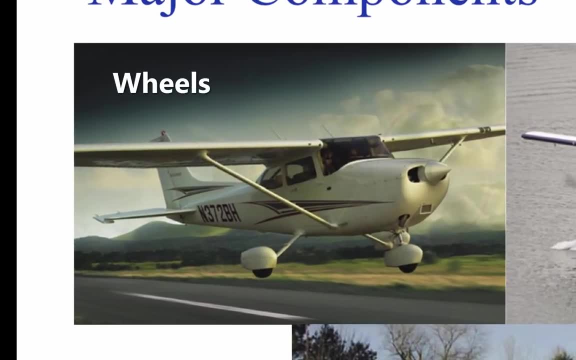 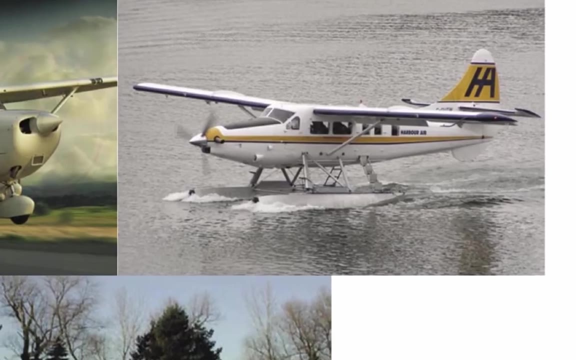 Landing gear are what support a plane when it is parked, taxiing, taking off and landing. The most common type of landing gear are wheels shown on the upper left. Planes can also be fitted with floats, pictured in the top right, which let planes land on water. 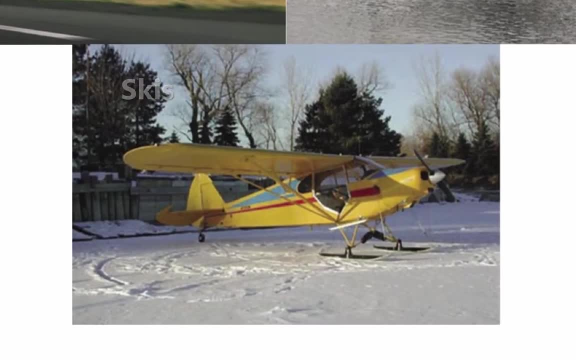 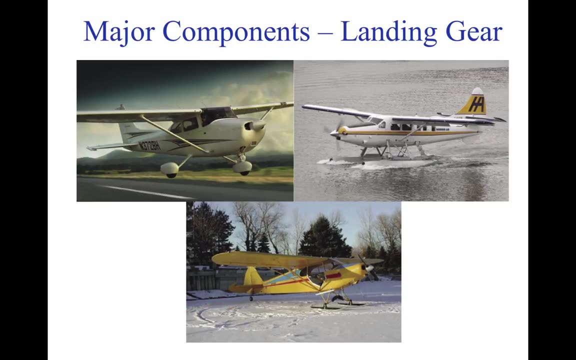 and skis pictured below are used to land on snow or ice. Airplanes with conventional landing gear are sometimes referred to as tailwheel airplanes. When the third wheel is located on the nose, it is called a nose wheel and the design is referred to as a tricycle gear. 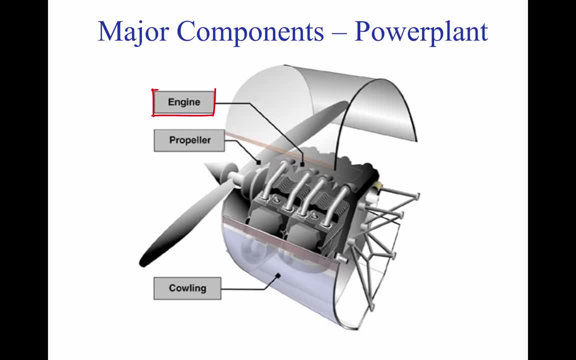 The power plant usually includes both the engine and the propeller. The primary function of the engine is to provide the power to turn the propeller. It also generates electrical power, provides a vacuum source for some flight instruments and, in most single-engine airplanes, provides a source of heat for the pilot and passengers. 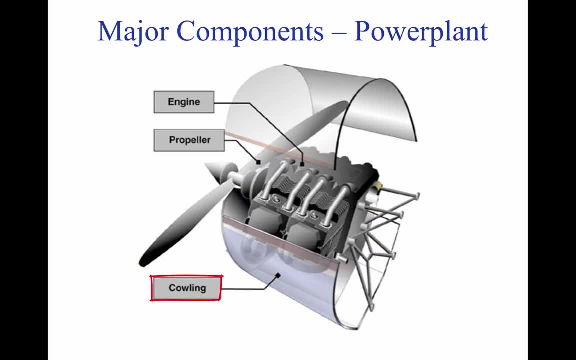 The engine is surrounded by a cowling, which makes the engine more streamlined and provides a way to duct air over the cylinders. The propeller mounted on the engine translates the engine's turning force into thrust. The propeller may also be mounted on the back of an aircraft and used to push the aircraft forward. 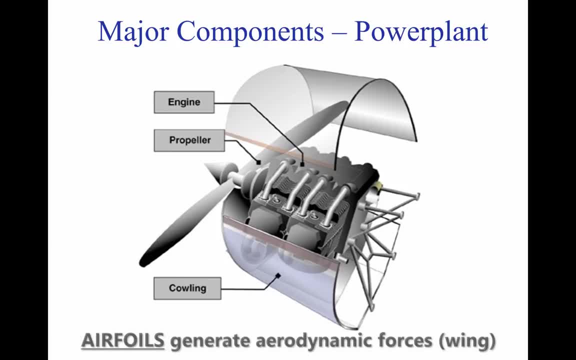 A propeller is a rotating airfoil that produces thrust through aerodynamic action. A low-pressure area is formed at the back of the propeller and high pressure is produced at the face of the propeller, similar to the way lift is generated by an airfoil used as a lifting surface or wing. 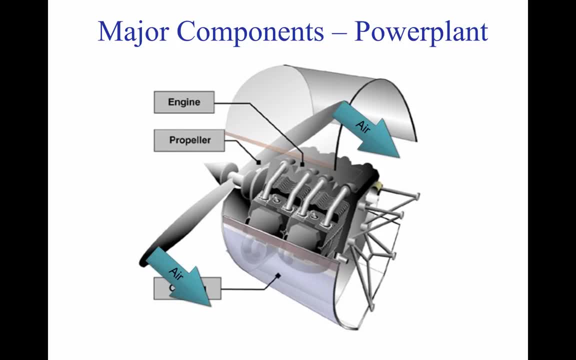 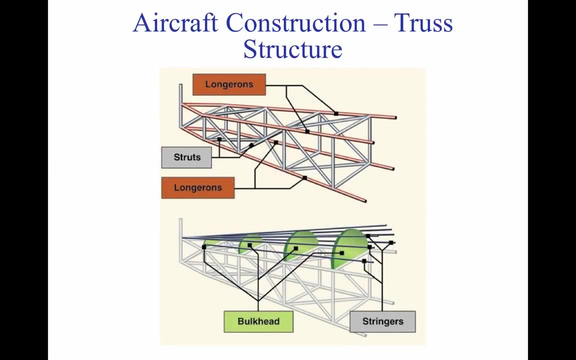 This pressure differential pulls air through the propeller, which in turn pulls the airplane forward. Aircraft have been made from all different materials, including wood, cloth, steel, aluminum and, more recently, composite materials. Pictured above is a fuselage made from a truss-style structure. 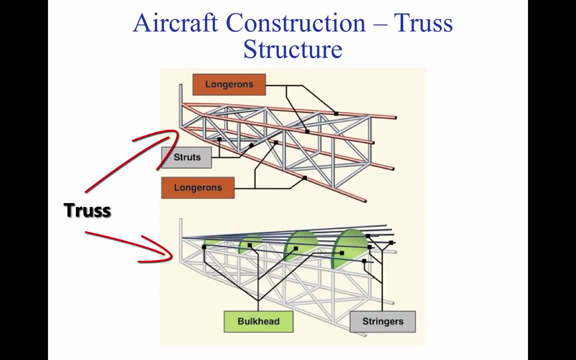 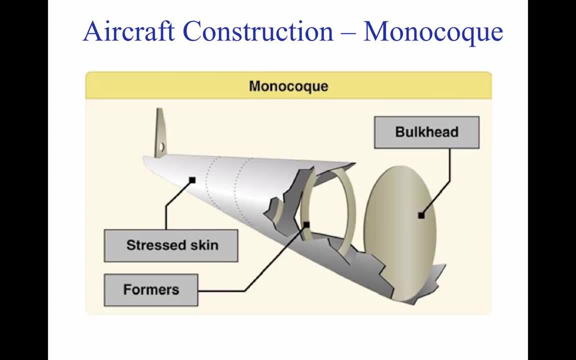 This design is not used very often because it lacks a streamlined shape. As technology progressed, designers started covering the truss members to make the aircraft more streamlined and have improved performance. Shown above is a monocoque fuselage design. This design relies on the skin of the aircraft to take most of the load. 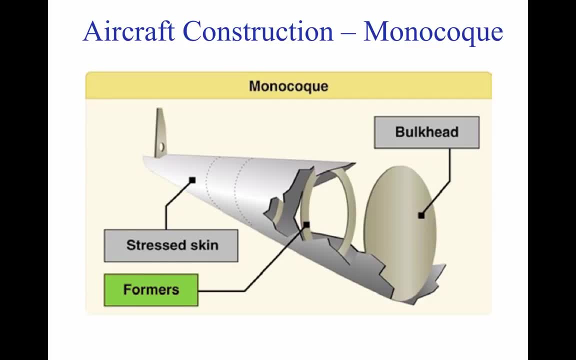 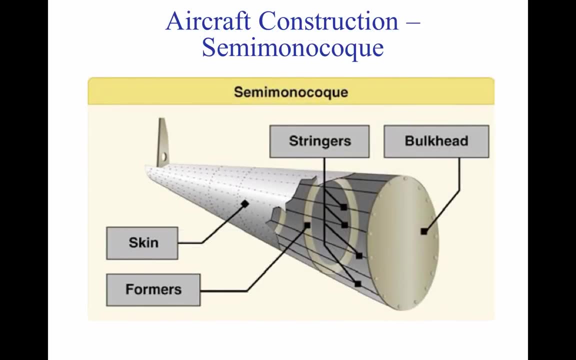 The skin is stretched over internal bracing and reduced the need for many struts inside the wing. This type of fuselage is designed to be used on the fuselage. This type of aircraft fuselage design combines the monocoque and truss designs and is called semi-monocoque. 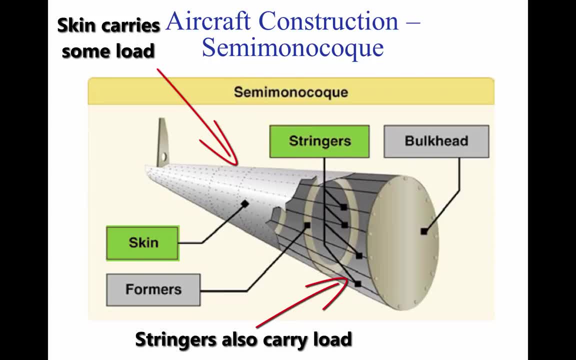 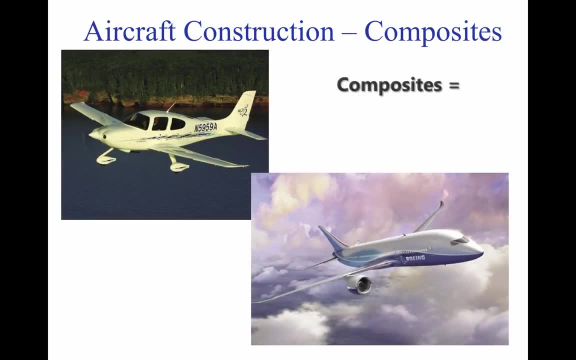 The skin still supports some load, while the stringers also carry load. This improves the strength of the fuselage over the monocoque design. Composite materials are fine fibers arranged in a matrix system held together by glue, such as epoxy and polyester resin. 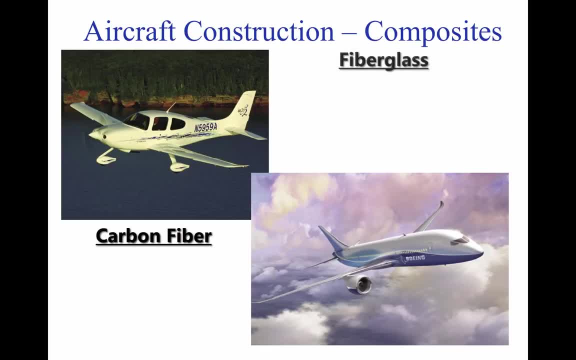 The fibers are most commonly made from carbon fiber or aluminum. The fiberglass has good tensile and compressive strength, good impact resistance, is easy to work with and is relatively inexpensive and readily available. Its main disadvantage is that it is relatively heavy and it is difficult to make a fiberglass load-carrying structure lighter than a well-designed equivalent aluminum structure. 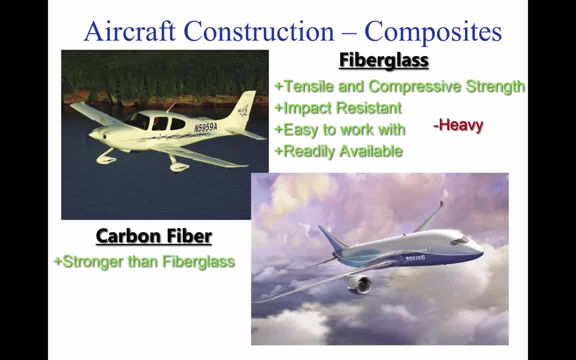 Carbon fiber is generally stronger in tensile and compressive strength than fiberglass and has much higher bending stiffness. It is also considerably lighter than fiberglass. However, it is relatively poor in impact resistance. The fibers are brittle and tend to shatter under sharp impact.